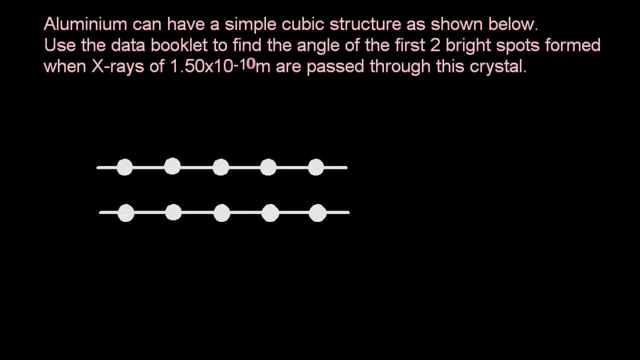 A simple cubic structure is all you need to apply this to in IV chemistry, and that means that the atoms are directly above each other in the planes in the crystal, just like the diagram here. So x-rays come in, x-rays go out, and we're going to use the Bragg equation, which is: n lambda equals twice times d the distance between the planes, sine theta. 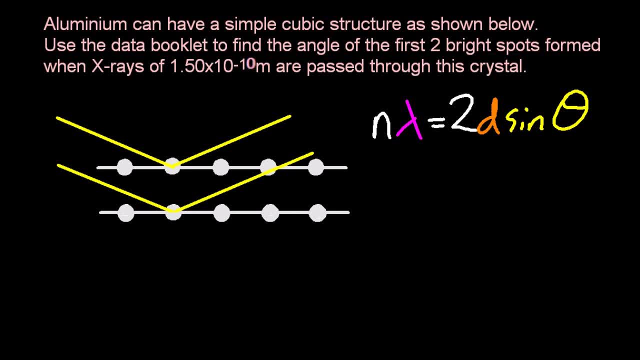 First two bright spots. well, that's n equals 1 and n equals 2.. Lambda is wavelength and there's the length, There, meters. You may have to convert to get to meters, but you need meters d. the distance between the planes is also the diameter of the atom. 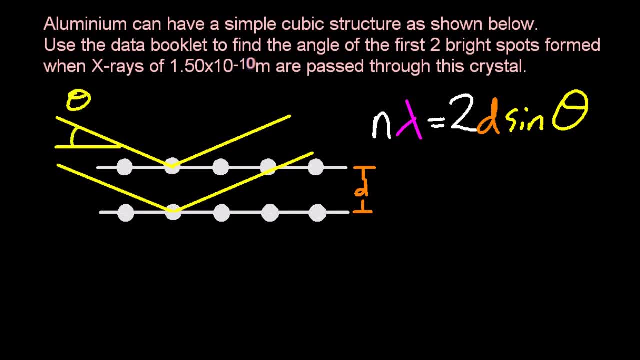 So you can look that up on the periodic table later. for the diameters or the radii, Theta is that angle there, And so let's just throw all the numbers in and see what we get. So setting n equals 1 for the first bright spot. 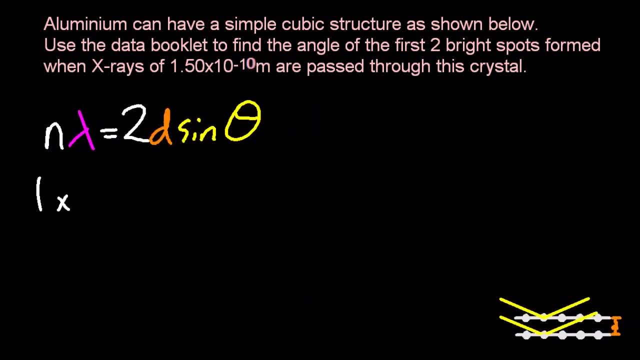 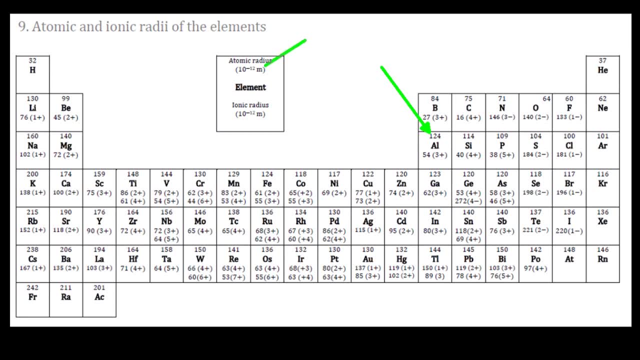 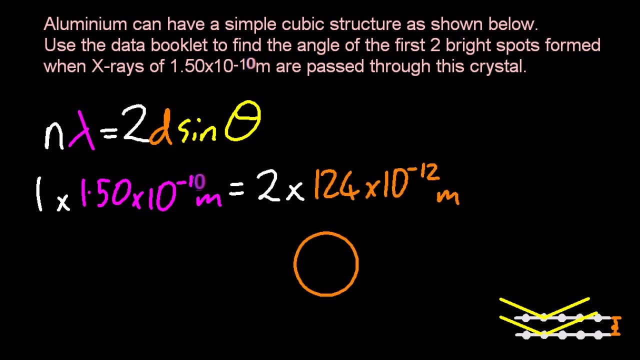 Multiply that by the wavelength Twice times, well, there's the radius of the aluminium atom. So I'm going to need the diameter d, so I'm going to need to double that Copyright IB, the data booklet, And multiply that by the sine of the angle theta. 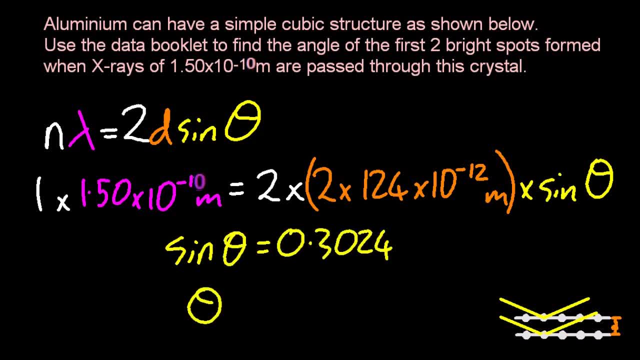 And that gets me the first angle of the bright spot. And that gets me the first angle of the bright spot And that gets me the first angle of the bright spot at 17.6 degrees, Three sig figs. And to get sine theta into the angle theta you probably have to use inverse and sine on your calculator. 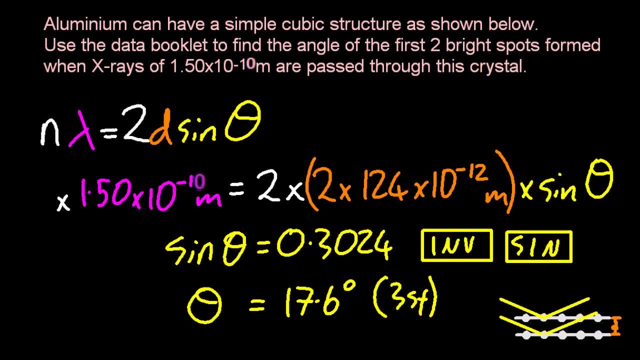 For the second bright spot, let's change n to 2.. Push all the numbers through again. Now I wonder if that's going to give me an angle twice as big. Nope, that's not how sines work. Nope, that's not how sines work. 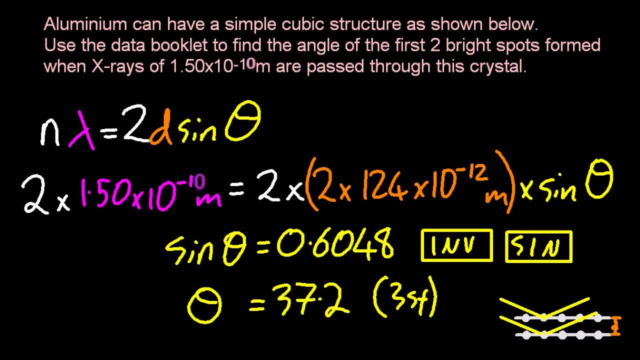 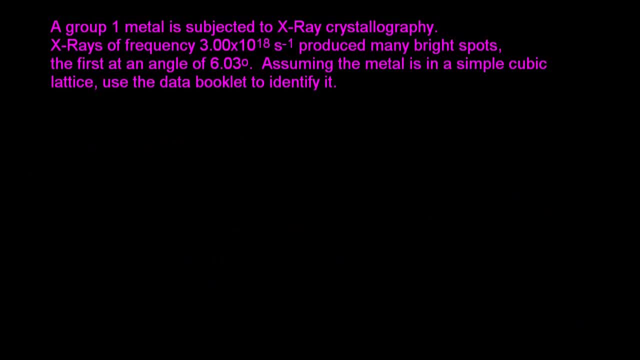 So the second bright spot, let's change n to 2. So the second angle is 37.2 degrees. Here's another question. So we're going to try to work out d the diameter of the atom, Then get r the radius of the atom.